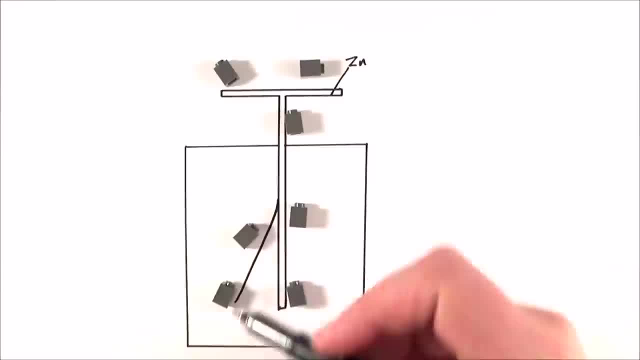 the charge left on this electroscope by the angle of the gold leaf. It's a bit like when you have a Van de Graaff and your hair sticks up and then cool the hair's repelling from the other hair. The same thing happens with the electroscope And what they found is if you put a load of red photons so you 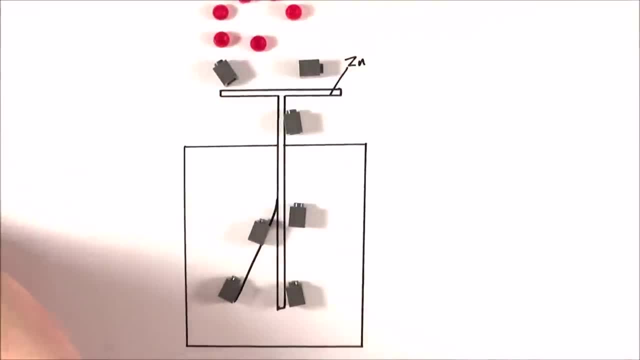 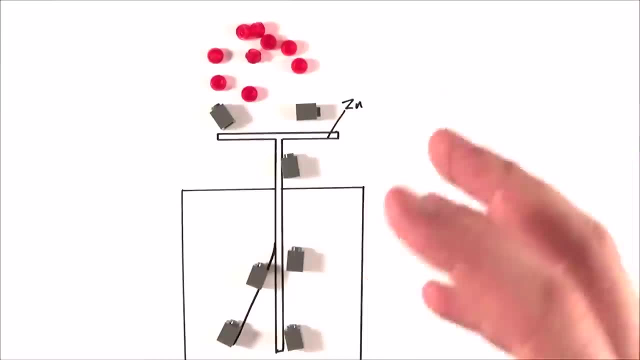 shone a load of red light at the zinc plate. nothing happened. You know you're just shining a load of red light at something. However, even if the radiation was very, very intense, you know there's lots and lots of bright light. 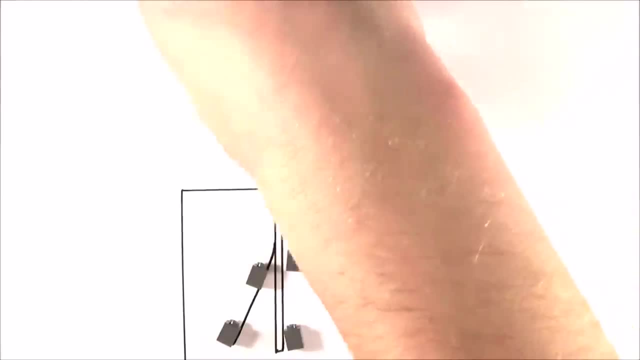 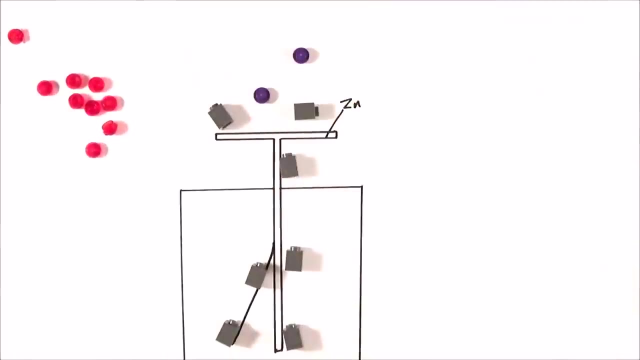 really very bright, nothing would happen. And they then found that if you just shone a small amount of ultraviolet- so here we have some of our ultraviolet photons sort of coming in the purpley coloured ones, even at very low intensities, these things here would somehow cause the electroscope to become. 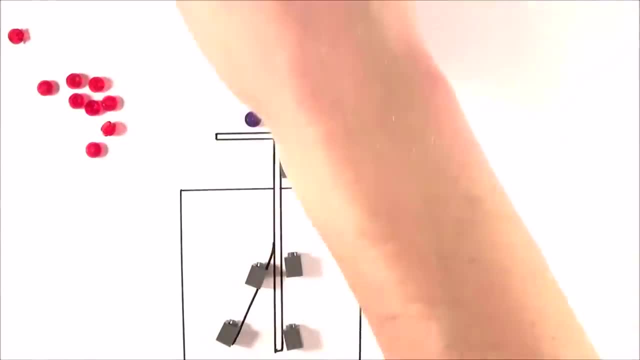 discharged And somehow these would cause the electrons to be emitted, And the more electrons are emitted, the lower the gold leaf would be. And this thing here was one brilliant example of the photoelectric effect. Certain photons would cause electrons to be emitted. However, they couldn't explain it. Why is it, if you've got the? 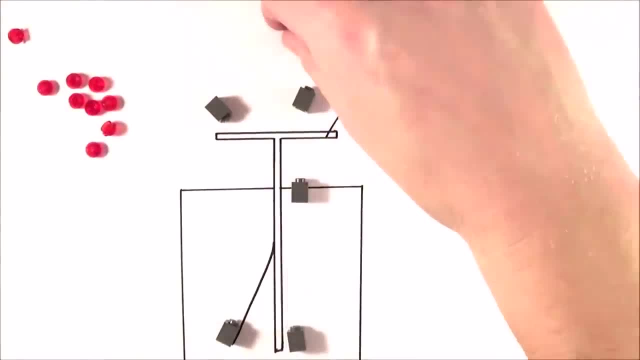 wave model of light. why is it? a couple of wavelengths of light or a few bits of light come in and they cause an effect to happen, Whereas you know by theory if you've got lots and lots of light on it, all the wavelengths, 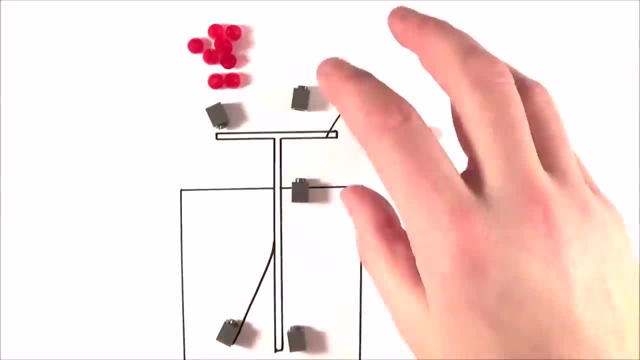 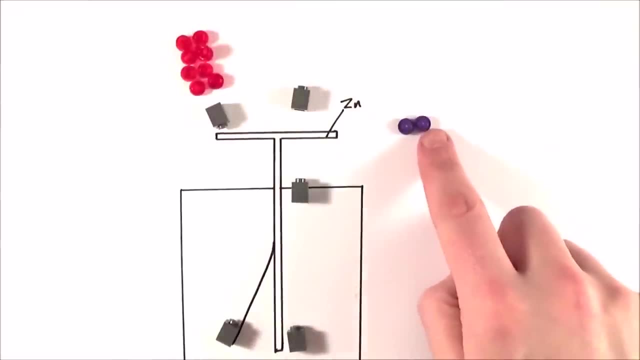 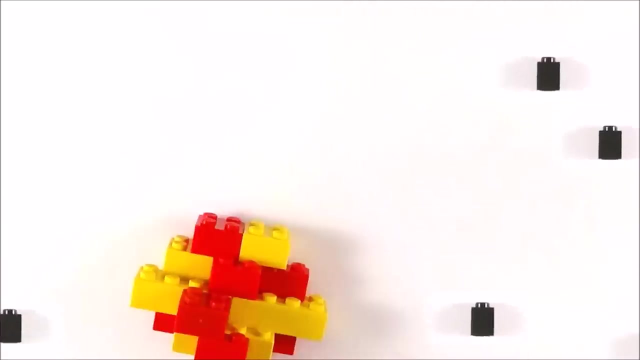 should combine together and in total give enough energy to get rid of these electrons. So the wave model could not explain how this happened, And it had to be something to do with the particulate nature of light, which is where Einstein came in. So here we have the model of the electron that we're used to. We have the kind of dense core surrounded by the various orbiting. 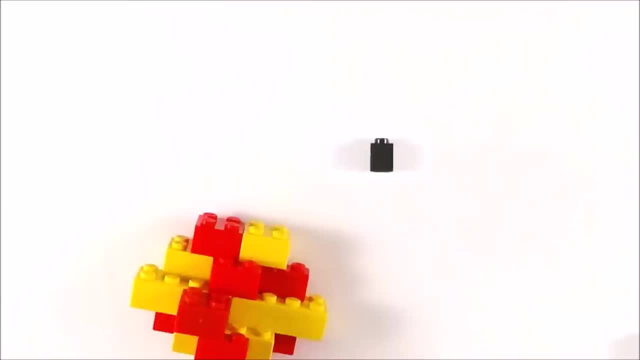 electrons in their shells, And what Einstein did was to really think about the electrons in those shells. In essence, this is what Einstein came up with. He had the idea that each of the atoms in its various shells with the electrons, in certain electrons are trapped within effectively. 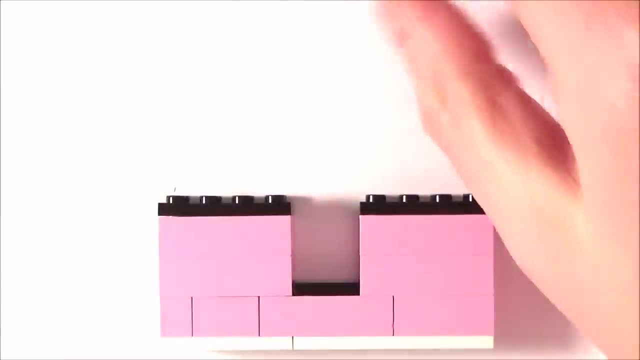 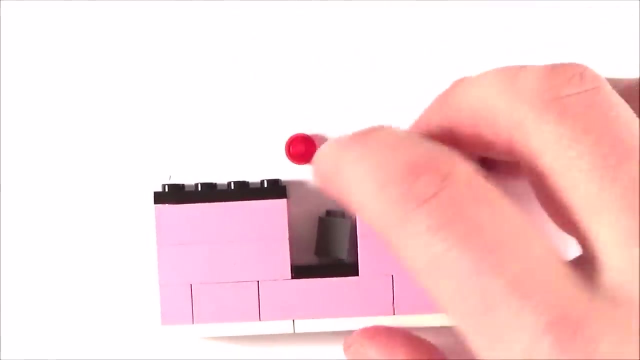 an energy. well, And in order to escape and actually be freed from that atom, this electron would have to absorb some energy. And if you had perhaps a red photon coming in, so a fairly low energy photon, it didn't have enough energy for this electron to absorb and then get away. 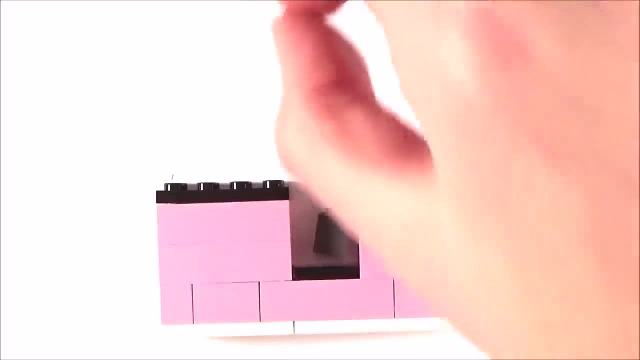 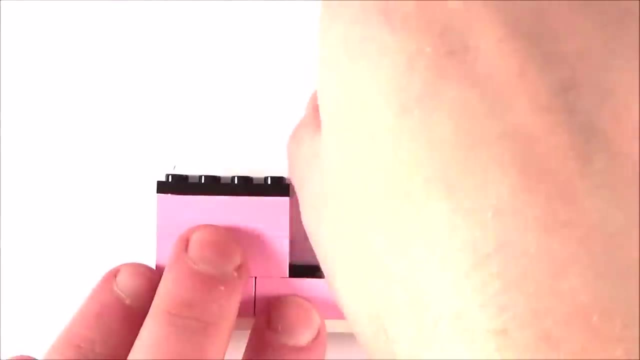 from the atom, And if it can't? if this photon can't be absorbed, then it won't be absorbed at all, And that means it just maybe just goes straight through past it. And if you have particularly highly energetic photons it's actually harder to do than I thought. 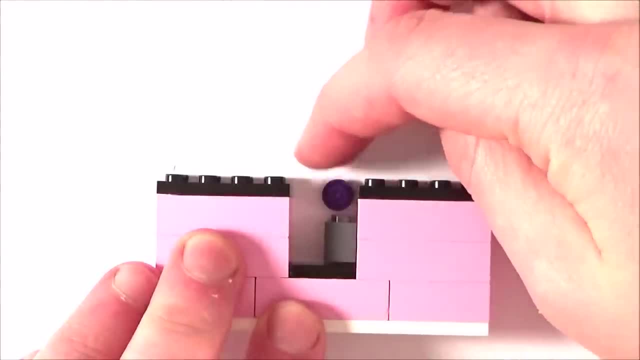 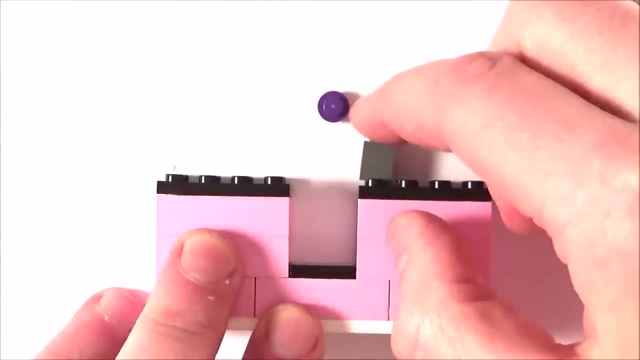 it would be If you have highly energetic photons, perhaps the ultraviolet. these ultraviolet photons are absorbed by the electrons. They move out from the energy. well, they overcome that the difference there, And then you might have some energy left after this has been. 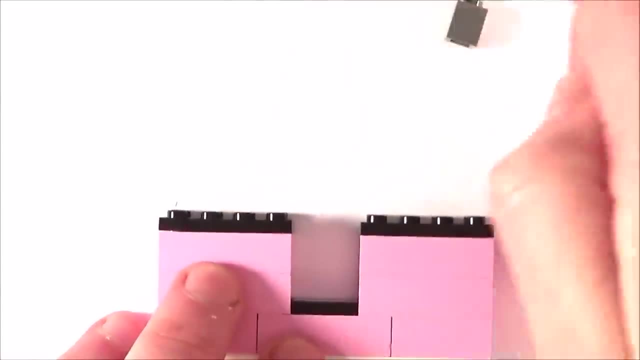 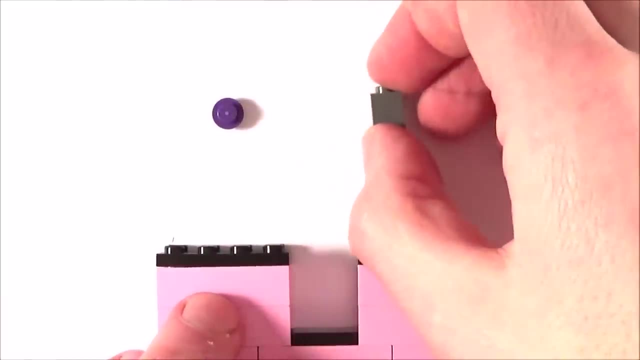 absorbed To then escape, And what we have is that the energy of the photon that's coming in is absorbed by the electron, It gets out of the atom and any energy left over is then converted into kinetic energy of this electron. And because this electron has absorbed a photon, 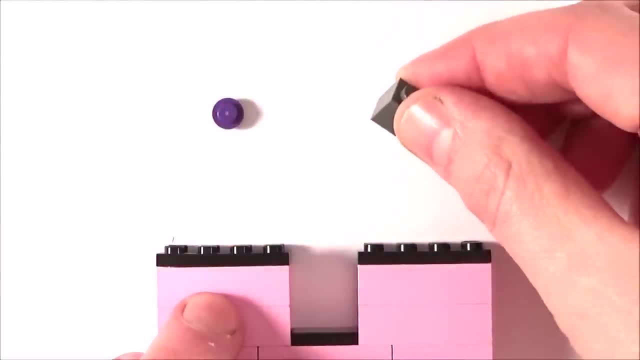 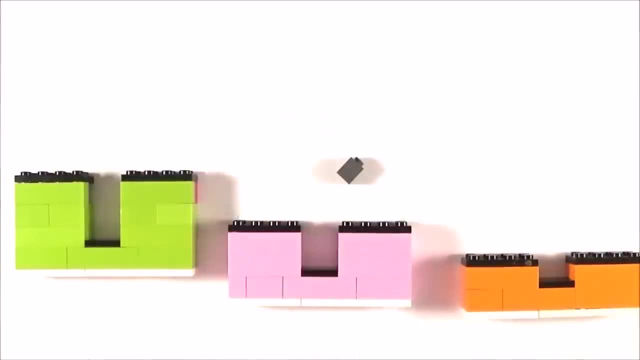 and is now moving away. this is called a photoelectron. Of course there's more than one kind of metal and different materials might have a different size energy. well, And what we find is that maybe, um some materials, they might allow the fairly low energy red photons to give them enough. 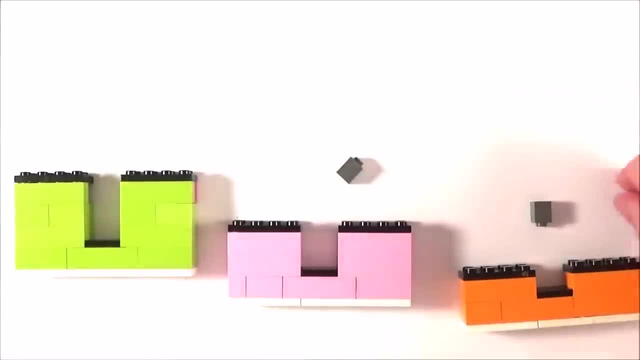 energy for the electrons to absorb the red photon, And then that allows these electrons here to then become photoelectrons. It might be that you have other, particularly tougher metals where you might even ultraviolet light might not allow the electrons to escape, And what we say is that each of these materials 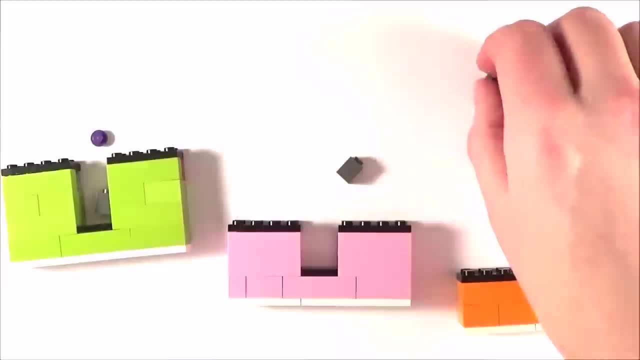 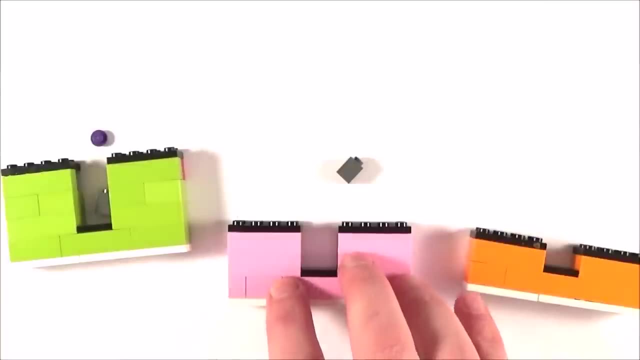 here has a different size energy. well, to actually get the electrons out, And we can give that a symbol, which is phi, And that stands for the work function. Okay, the work function is the amount of energy needed for the electrons to escape that energy. well, So what? Einstein? 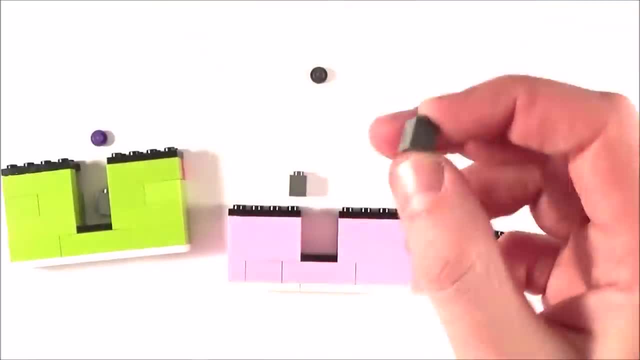 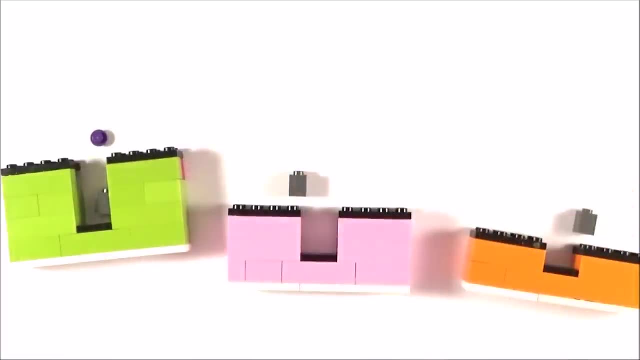 did was he explained why it is that these photoelectrons can only be emitted by photons that had a certain energy, And he put it all together into Einstein's equation, which I'll talk about in the next video. But it was really the only way to explain this was by using